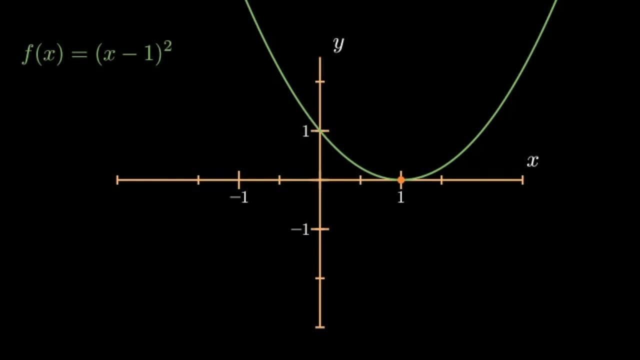 1, so it has a multiplicity of 2.. If we look at the graph of x squared plus 1, however, there's no real number that we could insert into this equation, such that f of x equals 0, no number squared plus 1 will give you 0, not for real numbers. So there seems to be some. 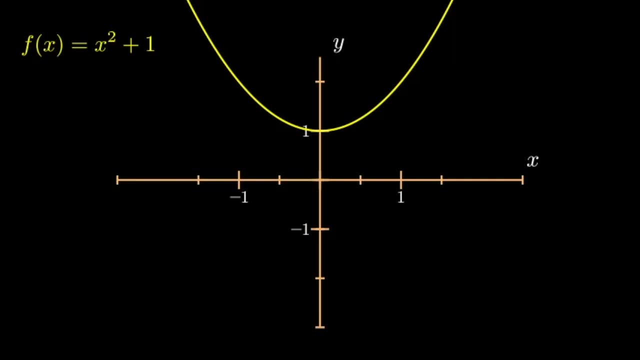 contradiction between the fundamental theorem of algebra and this quadratic polynomial. It turns out that we need a larger number system. We need to include the square root of minus 1, which we denote by i. So we'll define the complex numbers to be the set of all: a plus i, b, where a and b are real numbers. So if we 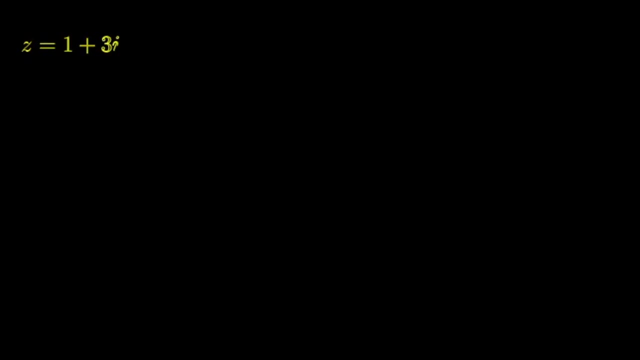 look at some specific examples of what a complex number is. we could take: z is equal to 1 plus 3i. The part that doesn't have an i in it, the part that has no square root of minus 1, we call the real part. So the real part of this complex. 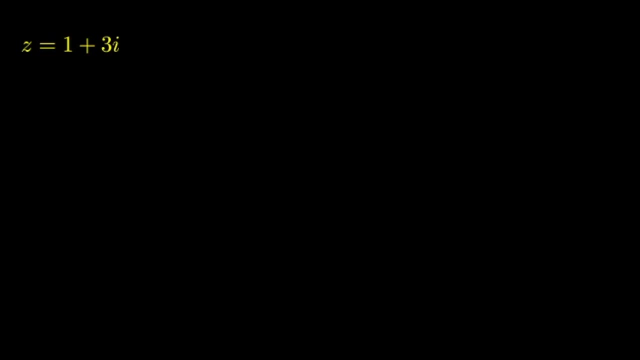 number is going to be 1.. The part with the i we call the imaginary part. So the imaginary part of this complex number is going to be 3.. If we just took the imaginary part to be 0, then we see that the real numbers form a subset of the. 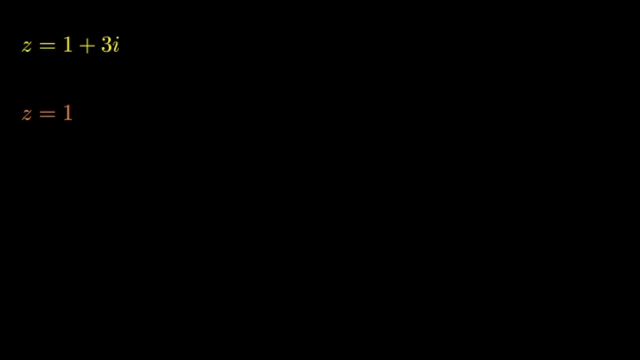 complex numbers, So any real numbers will be 0.. So any real number, such as z equals 1 can be taken to be a complex number also. Okay, so let's look at this first example. Let u equal 1 plus 2i and v equal 3. 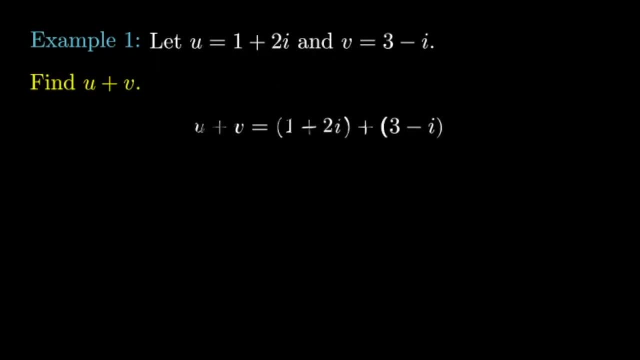 minus i. We want to find u plus v, So let's write u plus v as 1 plus 2i plus 3 minus i. We will remove the brackets and now we will just combine the real and imaginary parts. We get u plus v is 4 plus i. 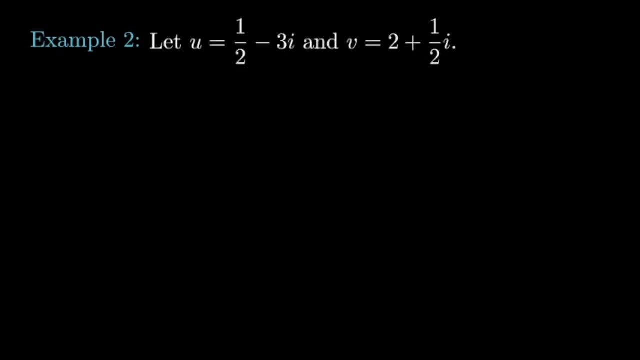 v is 1 half minus 3i and v is 2 plus 1 half i, And we will try to find u minus v. So again, we will write it as 1 half minus 3i minus 2 plus 1 half i, And we will just. 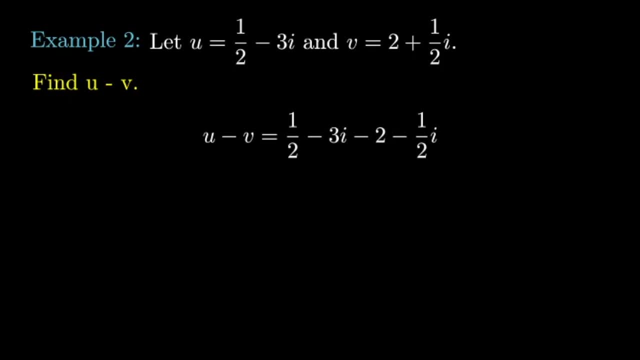 remove the brackets again. Now, if we combine the imaginary and the real parts together, we have 1 half minus 2, and then minus 3i minus 1 half i, And then if we add that together we just have minus 3 halves, minus 7 halves i. 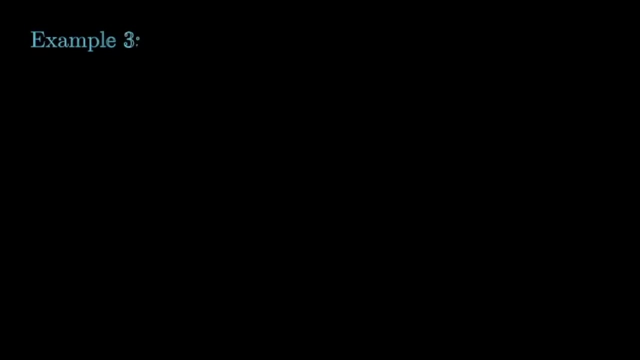 Let's look at a third example now. Let u equals 3 minus 2i and v equal 1 plus 6i. We want to find u times v, So again write u times v as 3 minus 2i times 1. 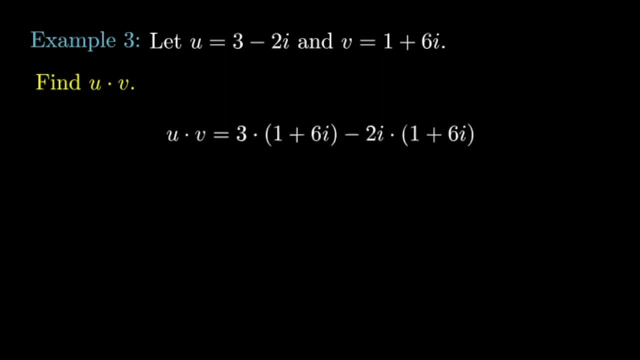 plus 6i, Then we can expand this as 3 times the first part minus 2i times the second part. So again, we can expand this as 3 times the first part minus 2i times the second part, And what we'll do is we'll just expand this 3 plus 18i minus 2i plus 12.. 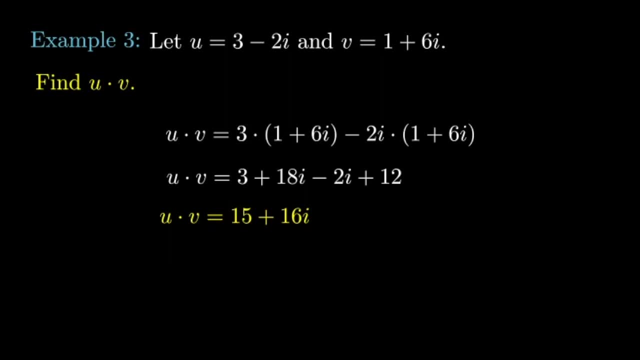 And then what we find is that u times v is just 15 plus 6i. Before we can talk about dividing complex numbers, we need to talk about complex conjugates. Given a complex number- z a plus i b- we will define the complex conjugate of z to be the complex number z a plus i b. 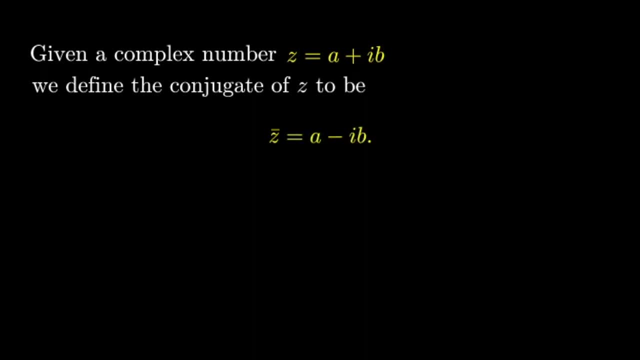 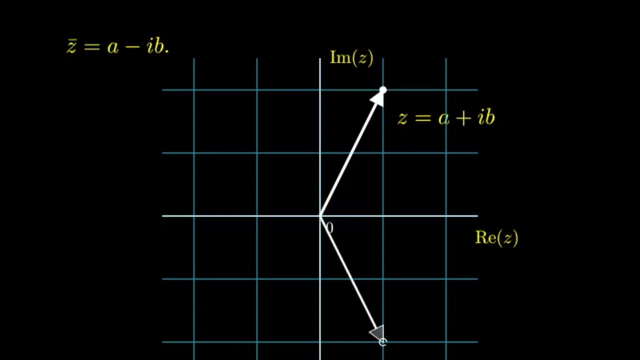 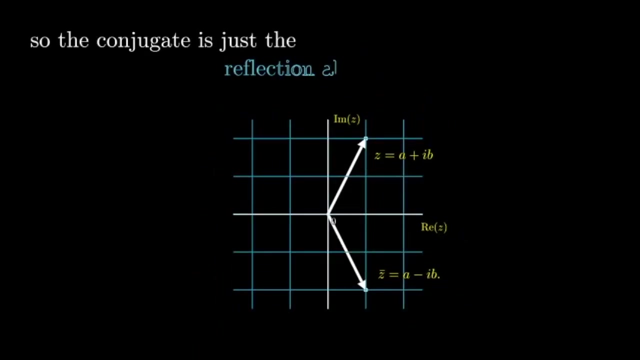 So if we were to look at this visually, if we graph, z is equal to a plus i b and the conjugate is going to be given by, z is equal to a minus i b and the conjugate is just taking the reflection of the complex number. about the real axis: 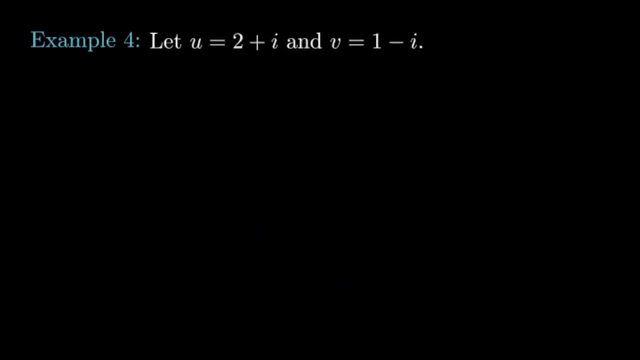 u is equal to 2 plus i and v is equal to 1 minus i. We want to find u divided by v, So we proceed in the usual way and write u over v is 2 plus i over 1 minus i. And what we're going to do is we're going to multiply by the conjugate of v divided. 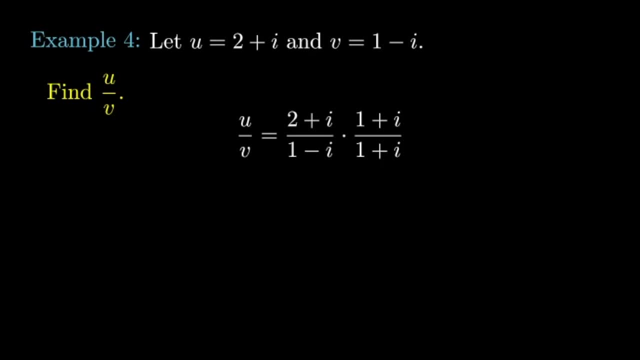 by the conjugate of v, Notice that this is just 1.. And then if we expand this expression, we see that we get 2 times 1 plus i plus i times 1 plus i. And if we expand the denominator we will just get 1 times 1 plus i plus i times. 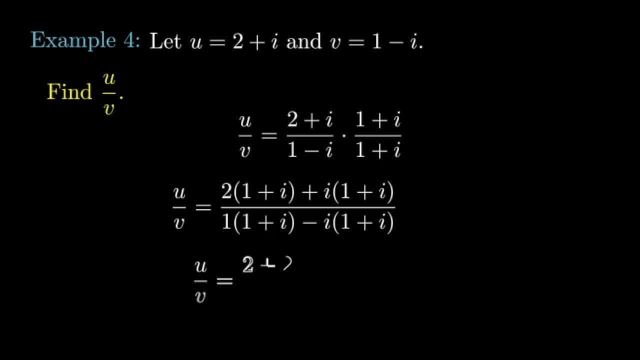 1 plus i minus. i times 1 plus i. Now, if we expand all this out, we'll get 2 plus 2i plus i minus 1.. And in the denominator we'll get 1 plus i minus i plus 1.. 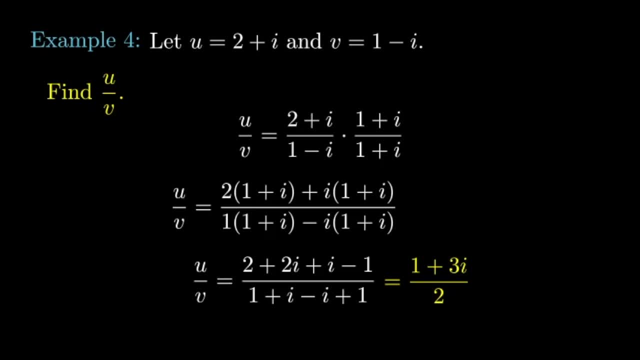 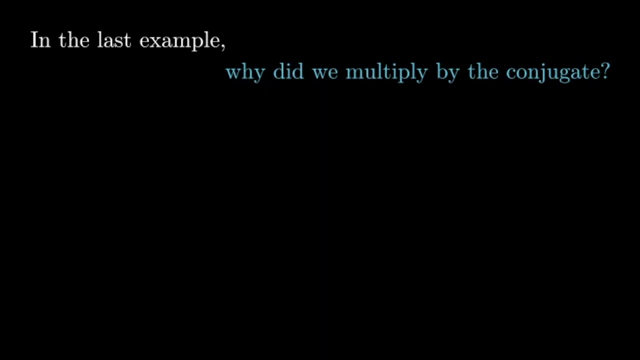 In the denominator we now have only a real part. So now, if we just simplify this expression, we end up with 1 plus 3i over 2.. So in the last example it's natural to ask why we multiply. Why do we multiply by the conjugate of the denominator? The main reason is polar coordinates. 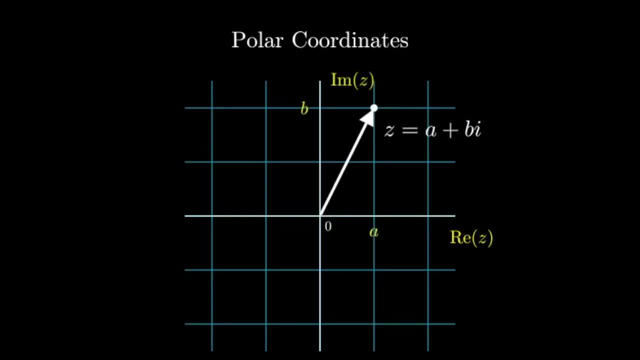 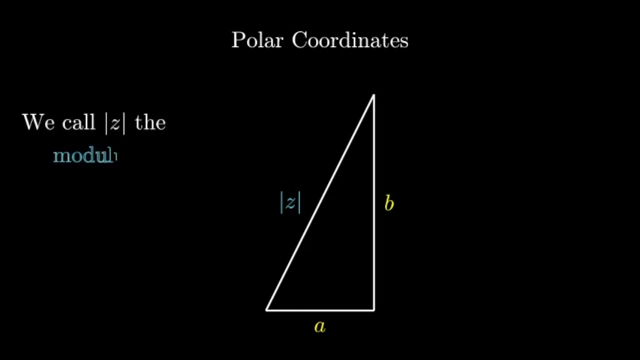 Let's draw our Argand diagram and we'll write our complex number. as z is equal to a plus ib, Form a triangle where the horizontal length is a and the vertical length is b. The length of this vector is now going to be given by Pythagoras And we call this length the modulus. 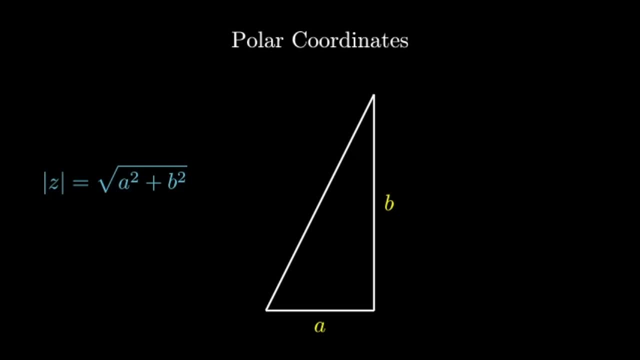 Now the modulus itself is not going to determine the complex number because I can have rotations, So I need to determine the angle between the horizontal axis and this complex number. That angle we call the argument From kindergarten trigonometry. sine is given by opposite over hypotenuse. 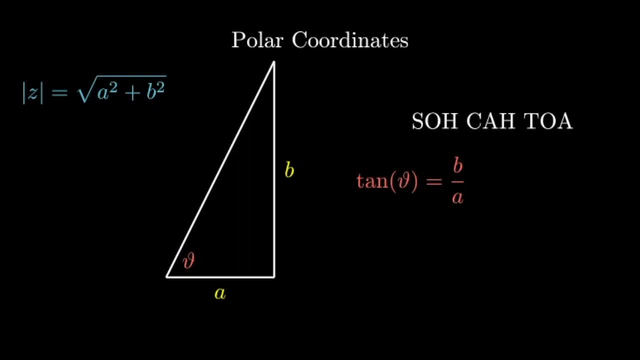 cosine is given by adjacent over hypotenuse. tan is given by opposite over adjacent. So our kindergarten mathematics says that tan of the argument, or tan theta, is equal to b over a. In other words, theta is given by the inverse tan of b over a. 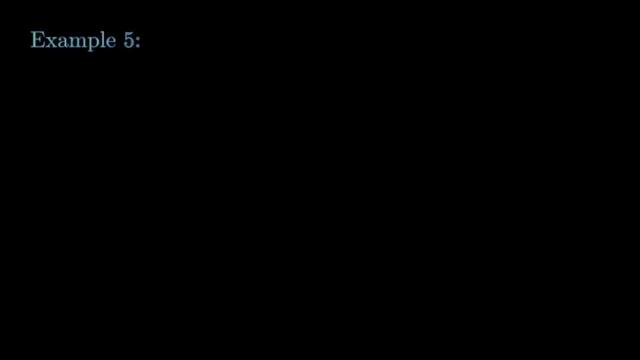 Let's now look at an example of converting a complex number into polar form. In this example, we'll convert z is equal to 1 plus i into polar form. Remember that polar form has two components: We need to calculate its modulus and we need to calculate its argument. 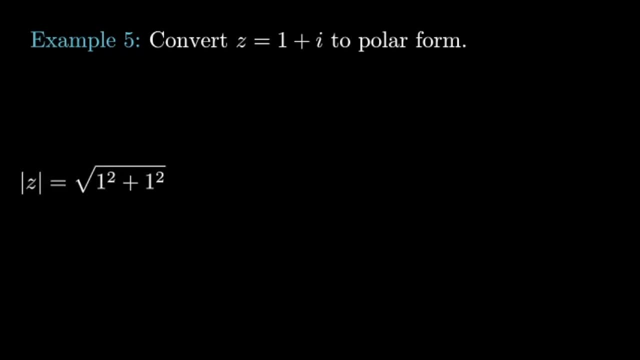 So the modulus is just going to be the square root of the real part squared plus the imaginary part squared. So the modulus of z is just going to be given by the square root of 1 squared plus 1 squared. In particular, the modulus of z is just going to be given by: 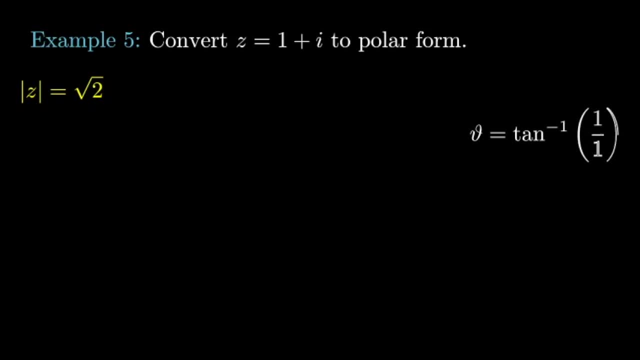 the square root of 2.. Now recall that to calculate the argument we need to calculate the inverse tan of the imaginary part divided by the real part. So we'll just get that theta is equal to the inverse tan of 1 divided by 1.. In other words, we'll have the inverse tan of 1.. The inverse 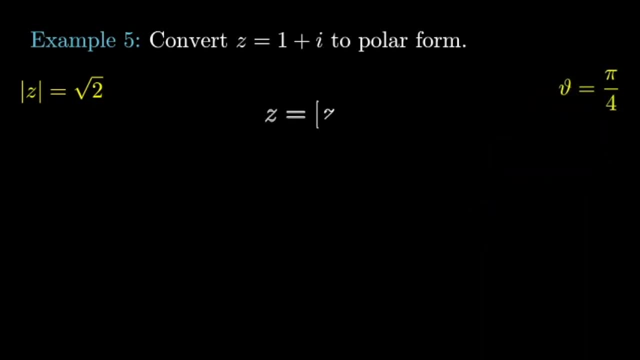 tan of 1 is just going to be the square root of 5 divided by 1 squared. So your basic formula is this going to be: pi on 4.. The complex number in polar form is mod z e to the i theta and so inserting: 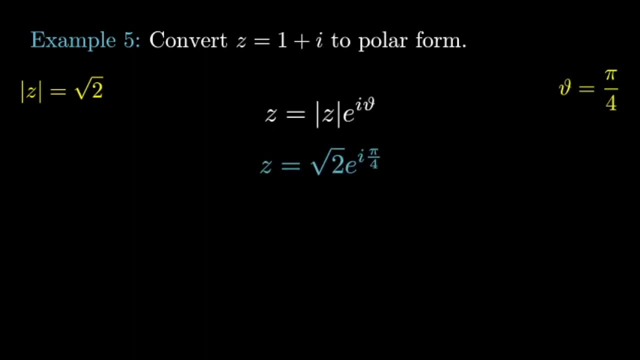 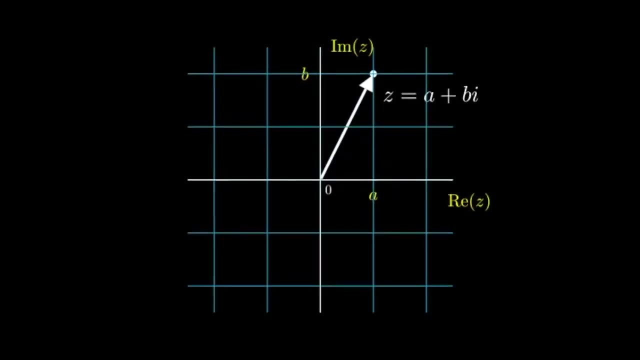 the values of the modulus and the argument, we find that z is equal to root 2, e to the i, pi on 4.. We'll draw our complex number: z is equal to a plus b, i, and what I can do is I can form the circle. 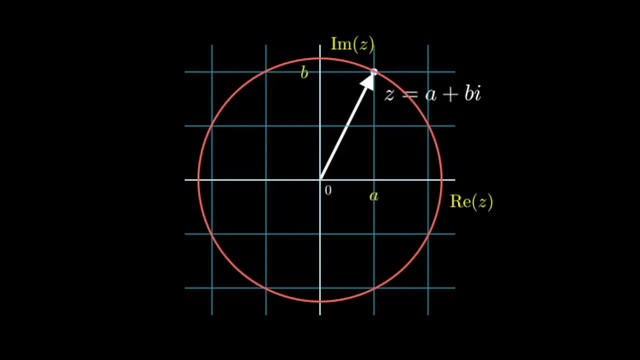 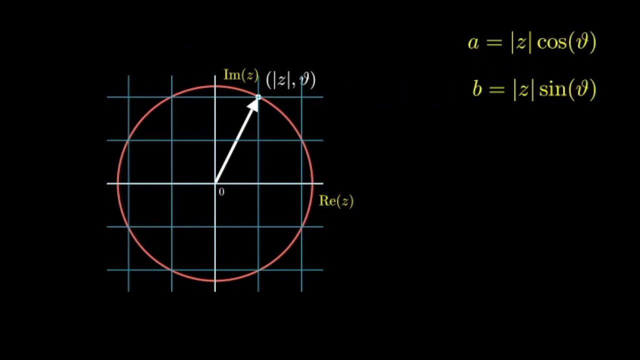 which is centered at the origin and has a radius given by the modulus of this complex number. So I want to replace a and b with the modulus and the argument. So what we see here is that the horizontal component is going to be given by mod z times cosine of theta, and the vertical 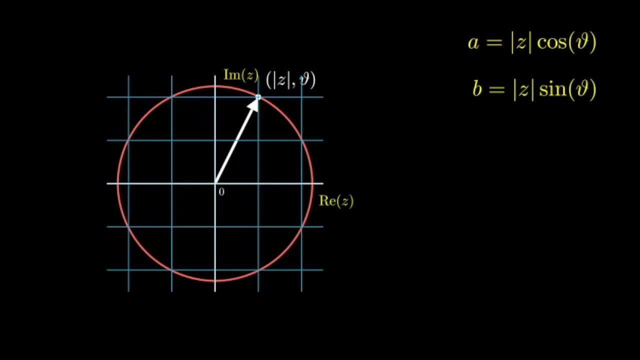 component is going to be given by mod z times sine of theta. So what I can now do is, instead of writing: z is equal to a plus b i. so what I can now do is write z as equal to mod z cosine theta plus i mod z sine theta. 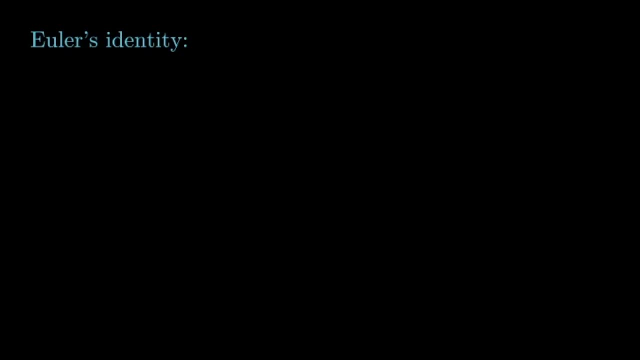 It turns out that there's a beautiful relation between exponentials and trigonometric functions that is bridged using complex numbers and that's called Euler's identity. Euler's identity says that e to the i theta is equal to cosine of the argument plus i sine of the argument. so 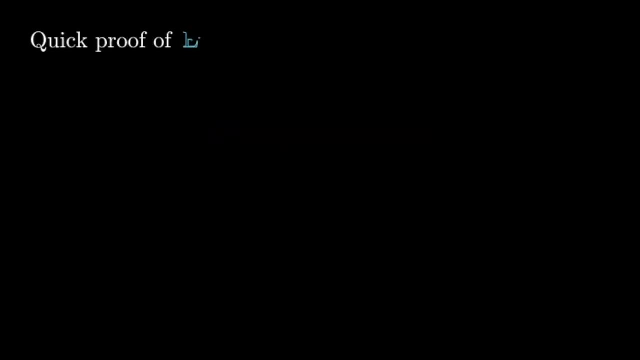 cosine theta plus i sine theta. So what we're going to do is actually give a quick proof of Euler's identity. So if we divide both sides of Euler's identity by e to the i theta, we find that one is equal to e to the minus i theta times: cosine theta plus i sine theta. 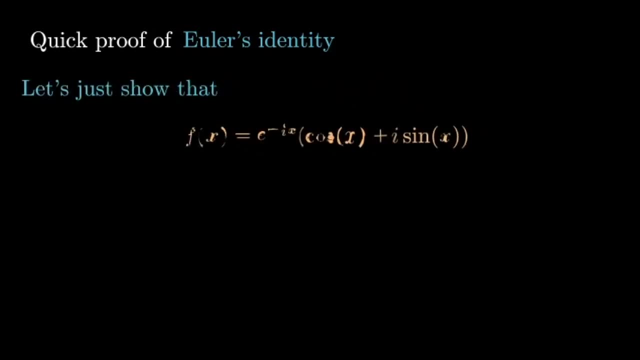 Let's define a function: f of x is equal to e to the minus i x times cosine x, plus i sine x. We need to show is that this is equal to one for all x. Now, one way we can do this is to just show. 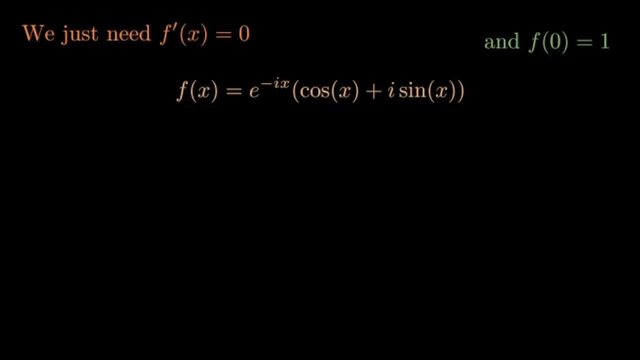 that the derivative is equal to zero everywhere and that initially it's equal to one. We find that x is equal to well. we'll differentiate the first factor and we'll get minus i e to the minus i x, and then we'll leave the second factor alone and have cos x plus i sine x, Now leaving the first. 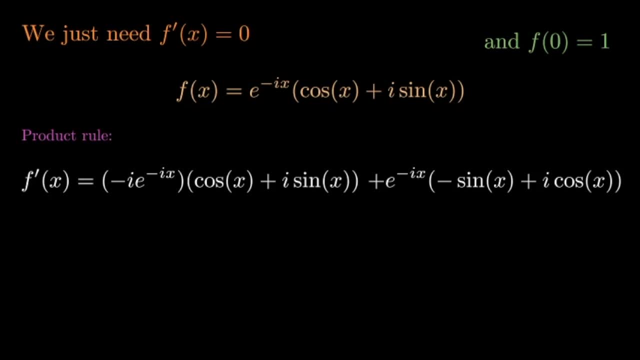 factor alone, but differentiating the second factor. we have sine x, but with a minus sign: plus i cosine x. Now, if we expand this first term out, we'll have e to the minus i x, minus i cosine x, squared sine x. Similarly, for the second part, we'll have e to the minus i x, minus sine x plus. 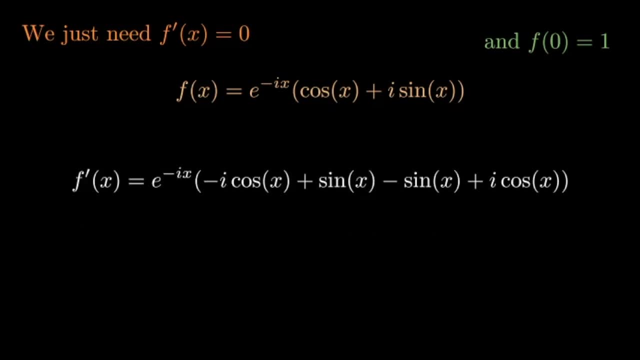 i cosine x, so nothing changes there. So if we combine all this together with e to the minus i x, out the front we'll have minus i cosine x, plus sine x, minus sine x plus i cosine x. that is equal to zero everywhere, because the cosines cancel and the sines will cancel. So now all we need to do is 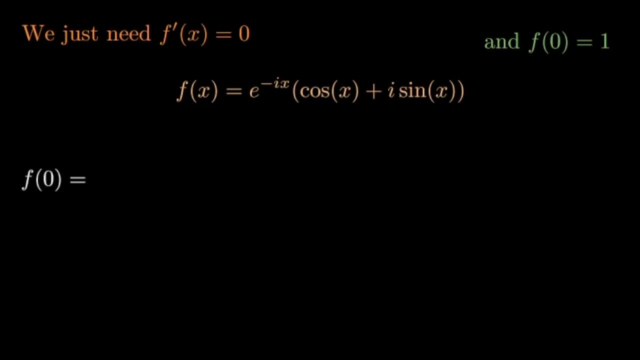 just show that f of zero is equal to one. Plug zero into this function. we get e to the minus i zero times cosine of zero plus i sine of zero. Now mickey mouse maths tells you that cosine of zero is one and sine of zero is zero. so we have e to the zero times one plus i. 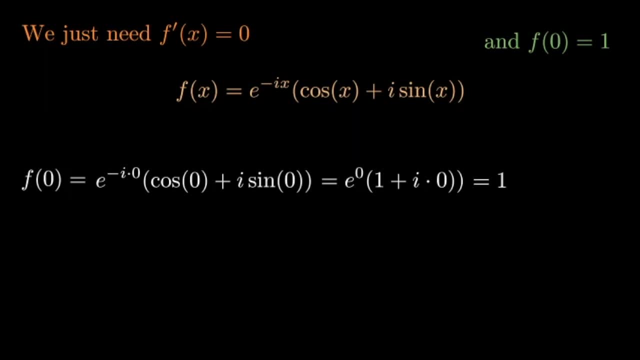 zero and the final answer is one. So that gives us a complete proof of Euler's identity. Since we're now familiar with complex numbers and the conversion to polar form, let's look at graphing of complex numbers, For example. let's look at: z is equal to one minus i. We want to analyze 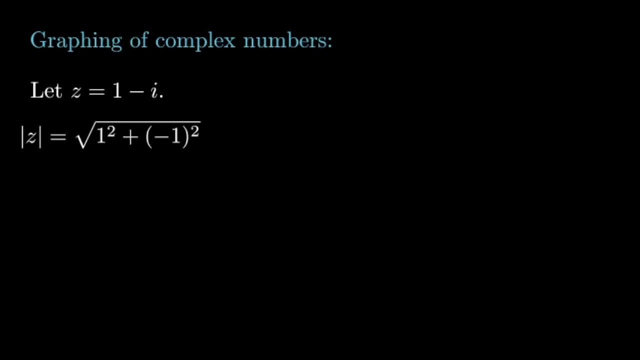 this in terms of polar coordinates. so what we'll do is we'll calculate the modulus and the argument. The modulus is going to be given by the square root of two. The argument is just going to be given by the inverse tan of the imaginary part over the real part. We'll have the inverse tan. 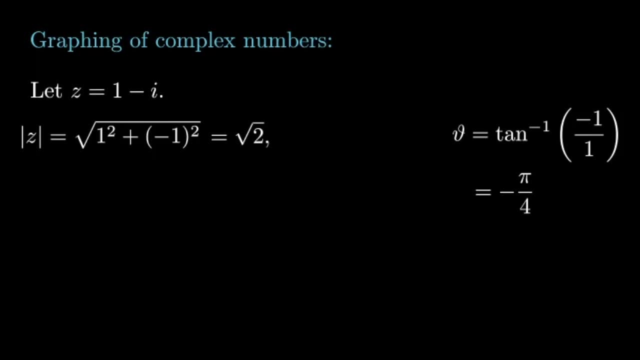 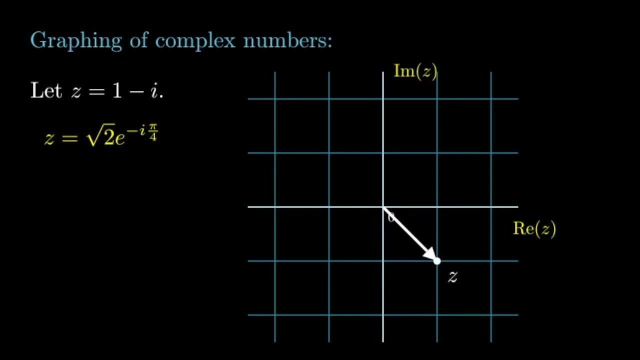 by one. so the inverse tan of minus one is just going to be minus pi on four, and so the polar form of the complex number is just root two times e to the minus i pi on four. So now visualizing this on an argand diagram or the complex plane: and so let's say we want to find minus z. So 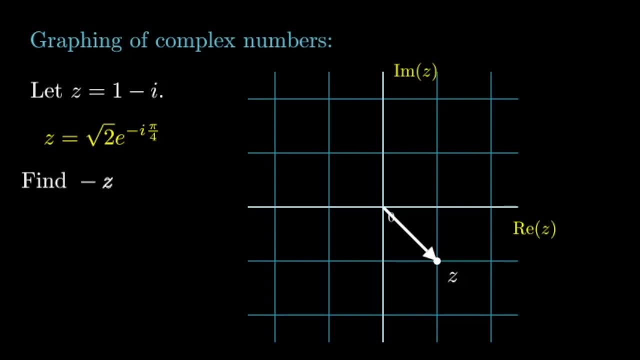 calculating it using the cartesian form we have: minus z is just minus one times one, minus i. that'll expand to minus one plus i and visualizing that on the argand diagram. And so what we see here is that it's a rotation anti-clockwise by 180 degrees and the corresponding 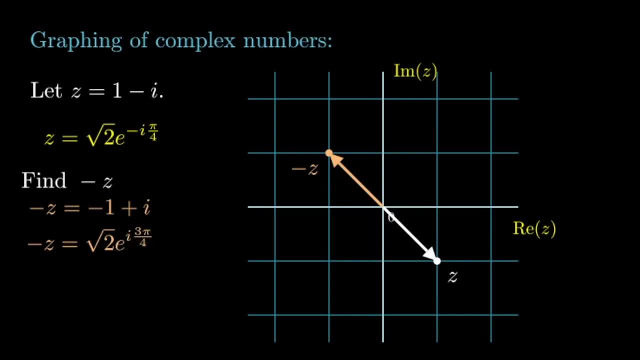 polar form. here is going to be root two e to the i, three pi on four Find i times z. So here, if we do it analytically using the cartesian form, we'll have i times one minus i. If we expand that out we 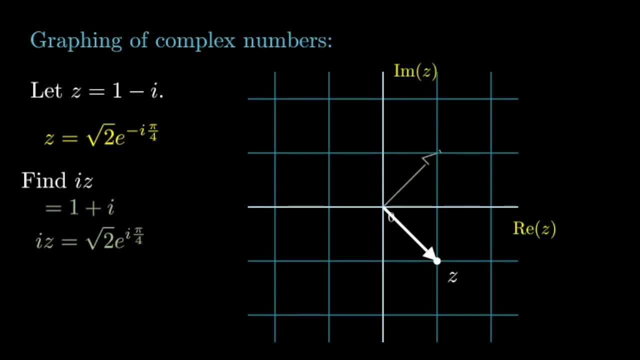 end up with one plus one minus one plus i. So if we do it analytically using the cartesian form, we'll have i times one minus i. If we expand that out, we end up with one plus i And we can visualize that on the argand diagram. In this case we see a few things: The argument, 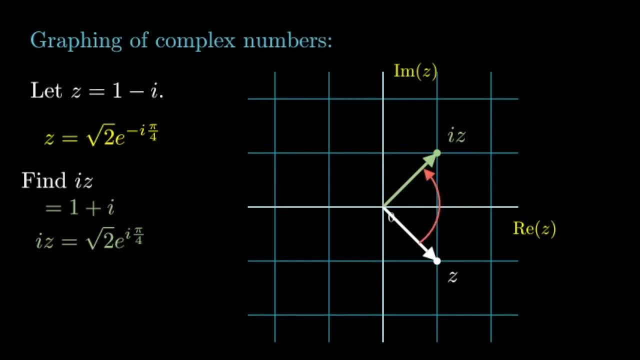 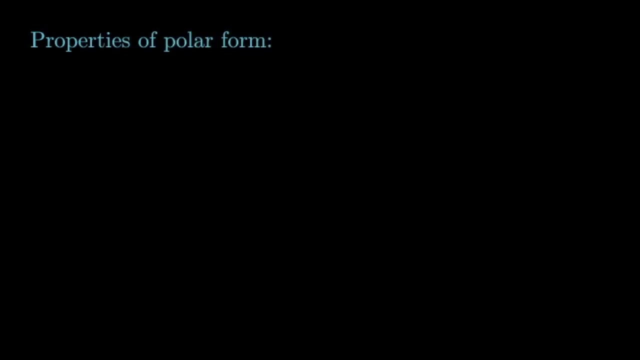 is now reversed. The main point here, however, is that when we multiply by i, the complex number you get when you multiply by i is a rotation by pi on two anti-clockwise. Since we now know Euler's identity, we can use the properties of exponentials to determine properties of. 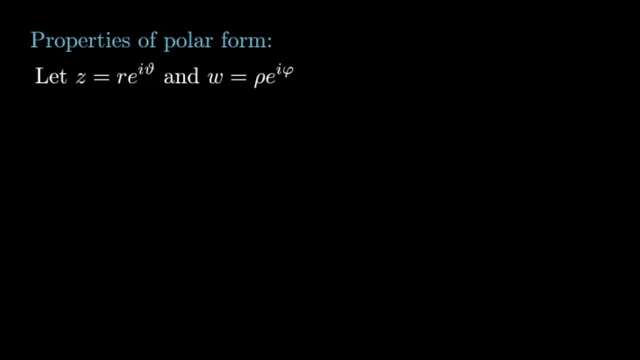 i. So let z equal r e to the i theta and w equal to rho e to the i phi. So r is going to be the modulus of z, rho is going to be the modulus of w, theta is the argument of z and phi is the argument of w. 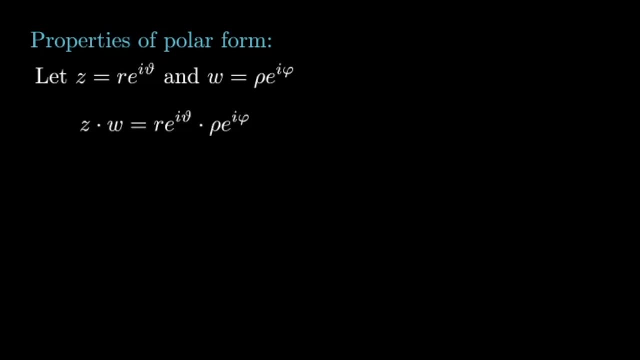 Now, if we multiply these two complex numbers, z times w, which is r e to the i theta times rho, e to the i phi, the moduli will multiply. so we'll just have r times rho and the exponentials we'll add. So what we'll have here is r times rho e to the i theta plus. 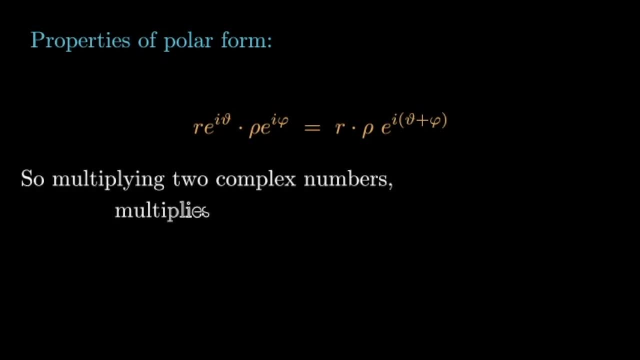 phi. The exponential laws tell us that when we multiply two complex numbers, we multiply their moduli and we add their arguments. Now we can do a similar thing with dividing complex numbers. So again, let z? equal r? e to the i theta and w equal to rho e to the i phi. Then z over w. 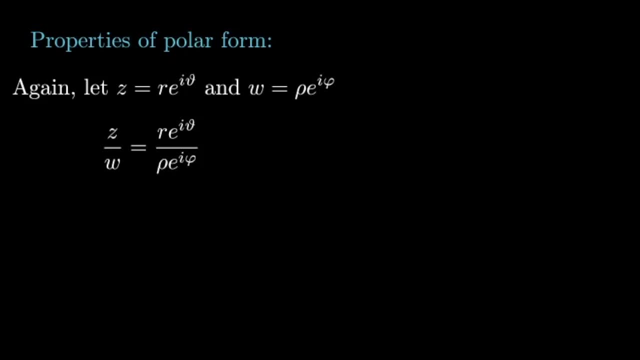 is r, e to the i theta divided by rho e to the i phi. So we'll end up with r divided by rho times e to the i theta minus phi. So again, dividing complex numbers divides their moduli and subtracts their arguments. So let's now look through another example, really combining all of these things, that 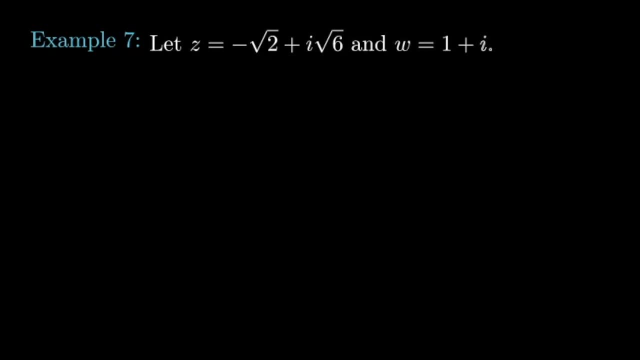 we've learned so far. Let z equal minus phi. We're going to hear the whole thing from here. If we root 2 plus i, root 6 and w equal 1 plus i, And we'll compute the ratio z over w. Let's just write: 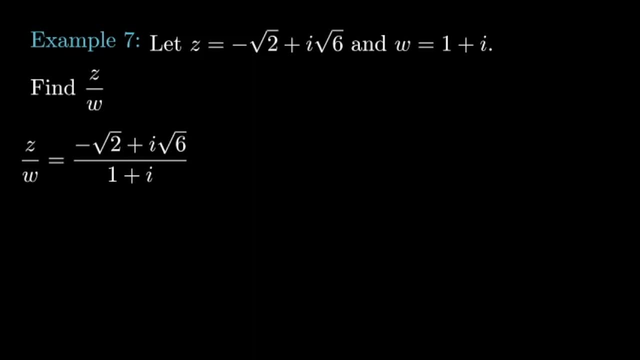 z over w is minus root 2 plus i root 6 over 1 plus i. As before, we'll multiply by the conjugate of the denominator and divide by the conjugate of the denominator. So now, if we expand this out, we end up with minus root 2 times 1 minus i plus i root 6 times 1 minus i, All divided by: 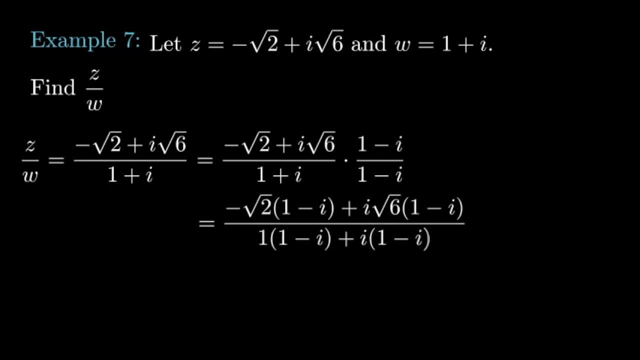 1 times 1 minus i, plus i times 1 minus i. So if we expand this out and collect the real and imaginary parts, we'll have minus root 2 plus root 6 plus i times root 2 plus root 6 over 1 squared. 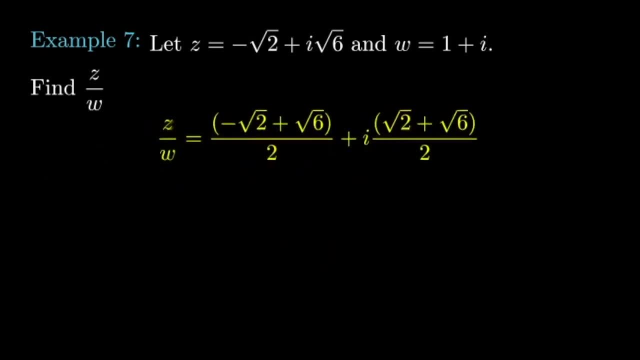 minus i squared, But that's just going to give us minus root 2 plus root 6 over 2 plus i times root 2 plus root 6.. So this time what we'll do is actually use polar form. So again we have: z is equal to minus root 2. 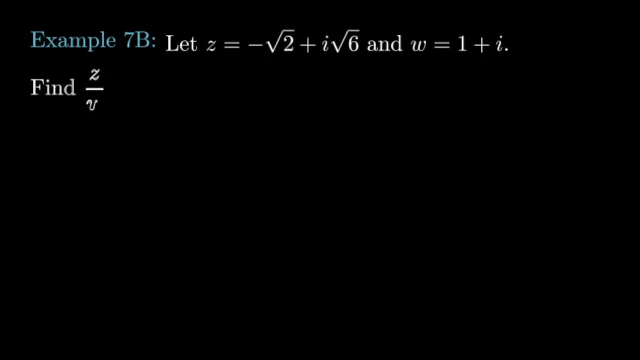 plus i root 6 and w is equal to 1 plus i. We want to find z over w. We have already computed their polar forms in previous examples. We have: z is equal to 2 root 2, e to the i 5 pi on 3 and w is: 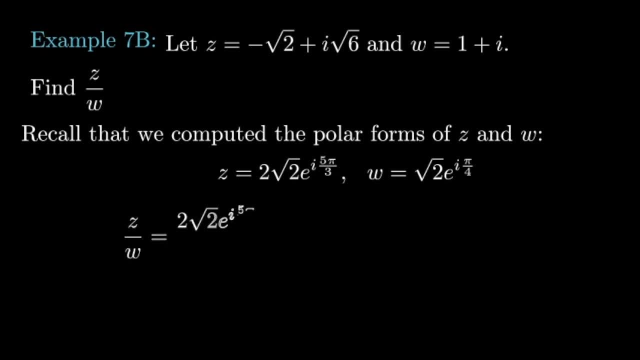 equal to root 2 e to the i pi on 4.. So now z over w is just going to be 2. root 2 e to the i 5 pi on 3.. So we're going to divide it by root 2 e to the i pi on 4.. So the root 2s are going to cancel. So 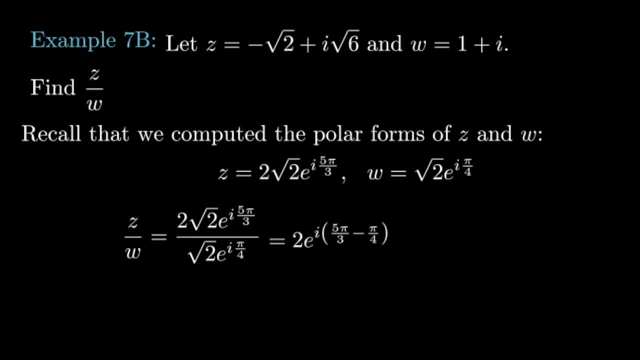 we'll have 2 e to the i, 5 pi on 3 minus pi on 4.. So when we simplify this fraction, we'll end up with 2 e to the i, 17 pi on 12.. Now, 17 pi on 12 is larger than pi. So if we wanted it in the 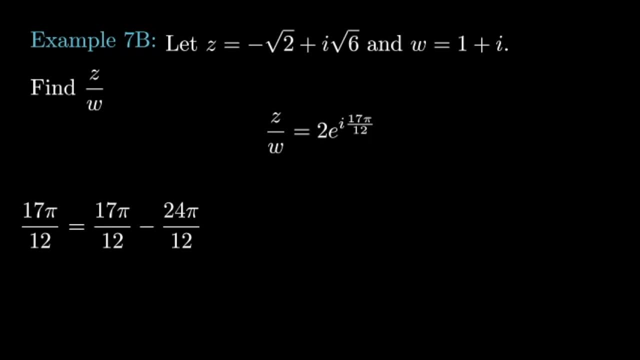 principal argument form, we'll need to subtract 2 pi. Now we can write 2 pi as 24 pi on 12. And then this just ends up being minus 7 pi on 12. Hence, in polar form z over w is just 2 e to the. 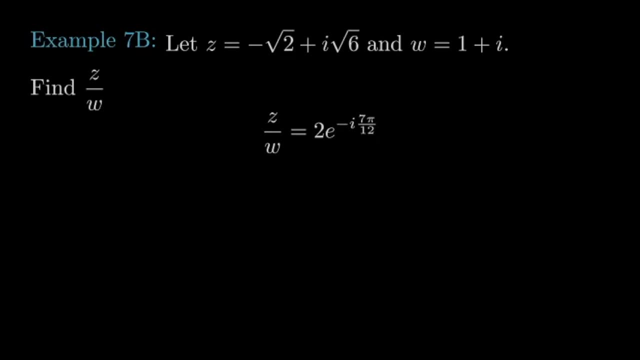 minus i, 7, pi on 12.. So one thing that's often very confusing is you calculate these complex numbers, You convert them into polar form and you find that the argument is not what the answer is in the back of the book. That's why we need to make the following remarks. So we'll draw a complex 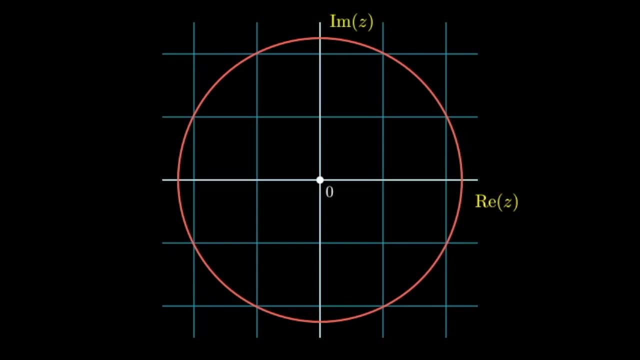 plane and we'll draw a complex plane. So we'll draw a complex plane and we'll draw a complex plane. We'll only look at complex numbers with the same modulus. Let's consider the complex number: z 1 is root 2 plus i root 6.. z 2 is minus root 2 plus i root 6.. z 3 is minus root 2 minus i root 6.. And 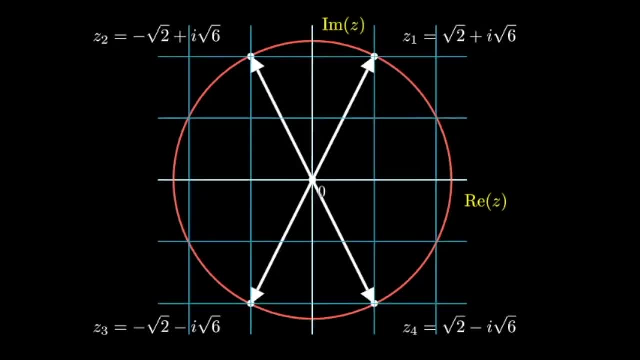 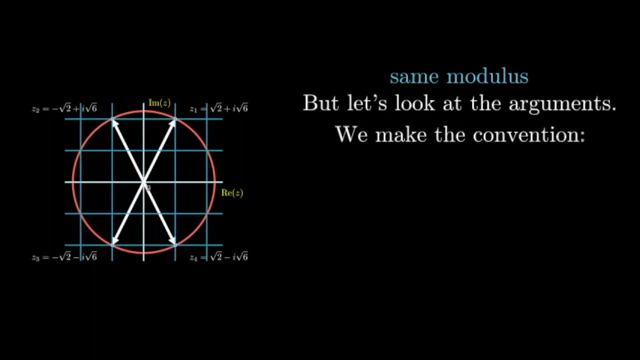 z. 4 is root 2 minus i root 6.. So all of these, you can check, have the same modulus, but their arguments will be different. The other thing we need to mention is that there is a convention Only take arguments that are between i and z. So if you have a convention that has a convention that has a 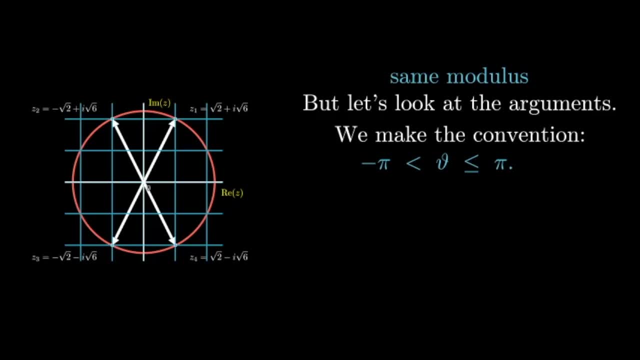 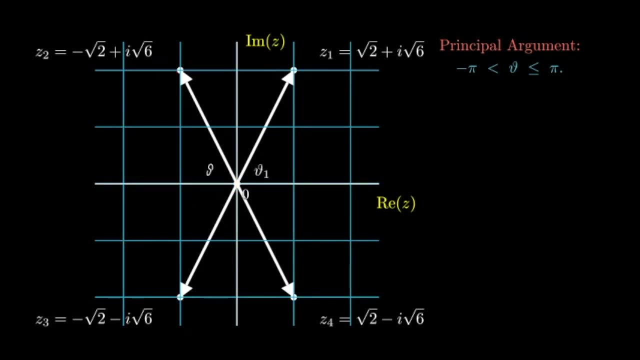 value between minus pi and pi, And so we call this the principal argument. So the negative real axis is going to be the boundary. So let's insert labels for the arguments. The argument of z 1 is going to be pi on 3.. The argument z to 2 is going to be given by going from pi and then subtracting. 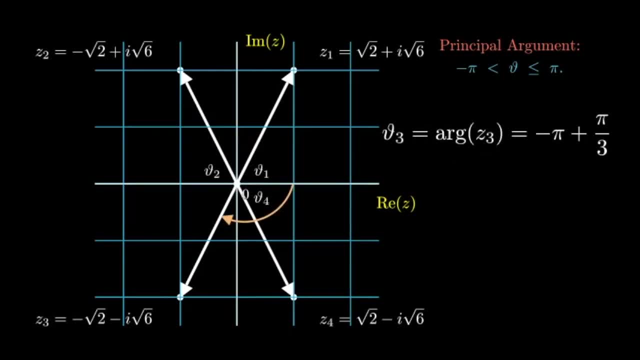 pi on 3.. The argument of z 3 is going to be given by going to minus pi and adding pi on 3.. And the argument of z 4 is just going to be minus pi on 3.. So we need to always make sure that the 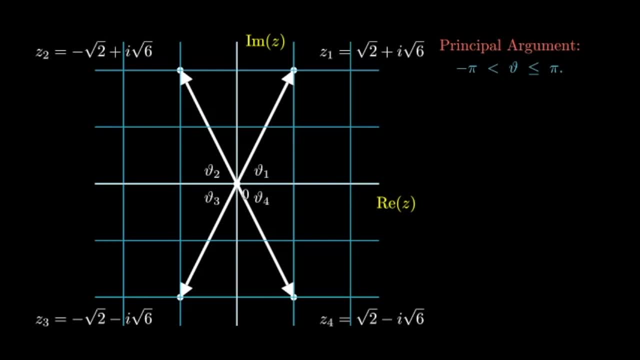 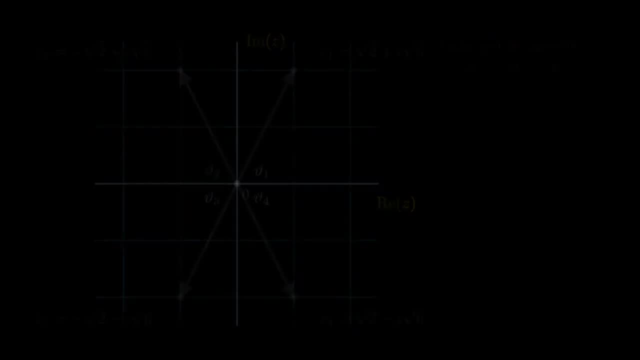 argument lies between minus pi and pi. If you end up with an answer that lies outside of that range, you have to add or subtract some multiple of two pi's. The one very nice application of complex numbers is that we can use complex numbers to find exact values of trigonometric functions. 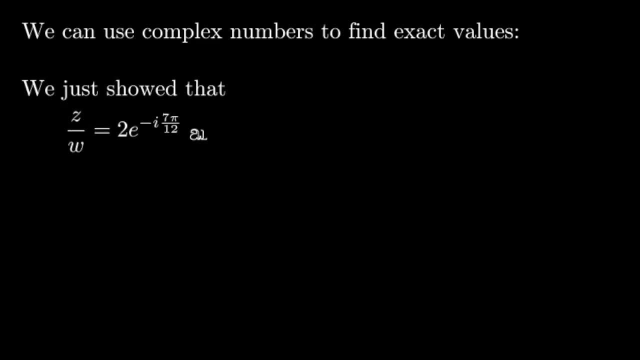 So we just showed that z over w is equal to 2e to the minus i 7 pi on 12.. And we also showed that z over w was minus root 2 plus root 6 over 2, plus i root 2 plus root 6 over 2.. We can go between polar form and cartesian form using 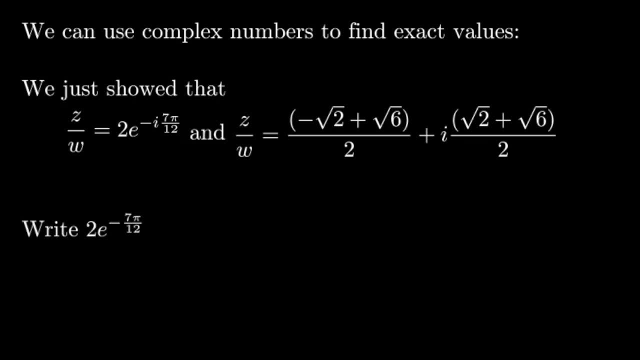 Euler's identity. We'll write 2e to the minus i 7 pi on 12 as 2 cosine minus 7 pi on 12, plus 2i minus 7 pi on 12.. So if we then write 2e to the minus i 7 pi on 12, we'll get 2e to the minus i. 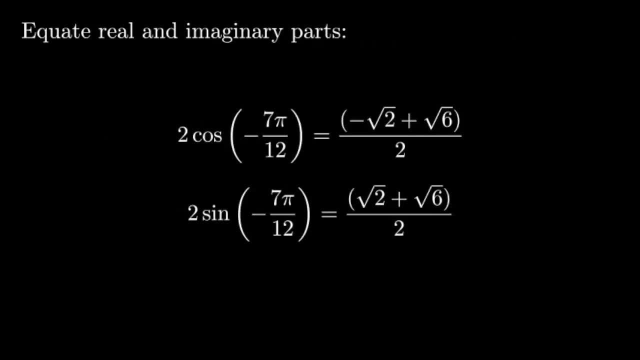 minus 7 pi on 12 plus 2i minus 7 pi on 12 plus 2i minus 7 pi on 12 plus 2i minus 7 pi on 12.. So we can equate the real and imaginary parts of these complex numbers. We'll have 2 cosine of minus. 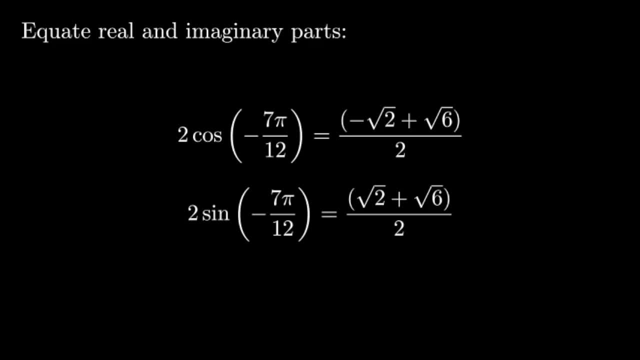 7 pi on 12 is equal to minus root 2 plus root 6 over 2.. And 2 sine minus 7 pi on 12 is equal to root 2 plus root 6 over 2.. Now cosine of x is even meaning that I can just get rid of the minus sign. 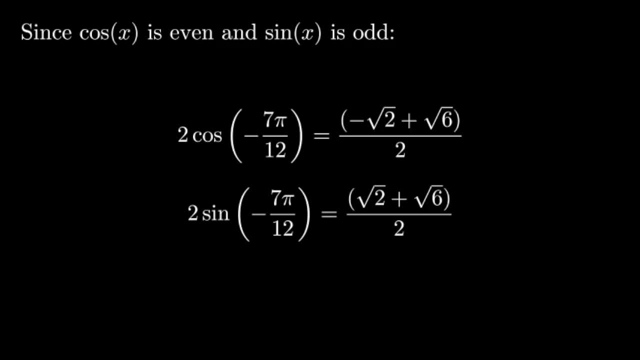 on the inside And sine x is odd meaning, I can just take the minus sign out the front, And so cosine of 7 pi on 12 as minus root 2 plus root 6 divided by 4.. And sine 7 pi on 12 as minus root 2. 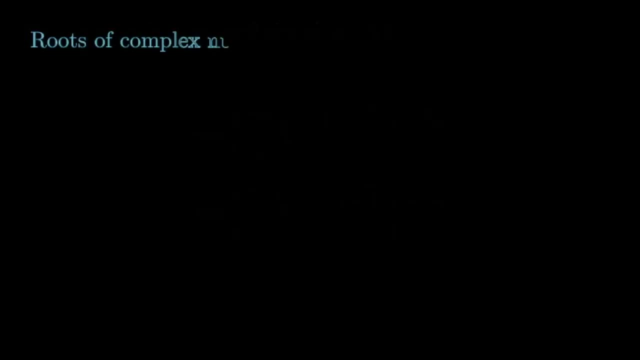 plus root 6 over 4.. So let's now take a look at taking the roots of complex numbers. So the first thing we want to look at is solving the equation. z squared minus 1 is equal to 0.. We get: z is equal to plus or minus 1.. 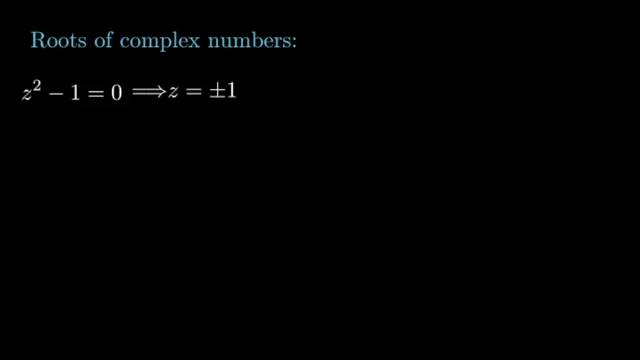 Gauss's fundamental theorem of algebra then tells us that these are the only roots of this polynomial. If we now visualize these roots on the Argand diagram, we have two points on the real axis, corresponding to minus 1 and 1.. Now let's suppose instead that we want to look at the cube. 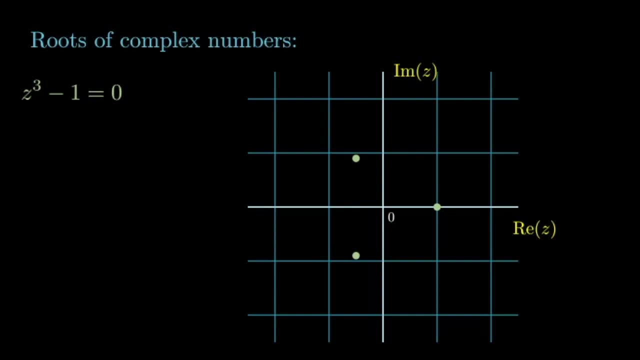 roots of 1.. And what we find is that we actually get three points. If we look at the four roots, we'll end up with 1 minus 1 i and minus i. If we look at z to the 5 is equal to 1, then the five. 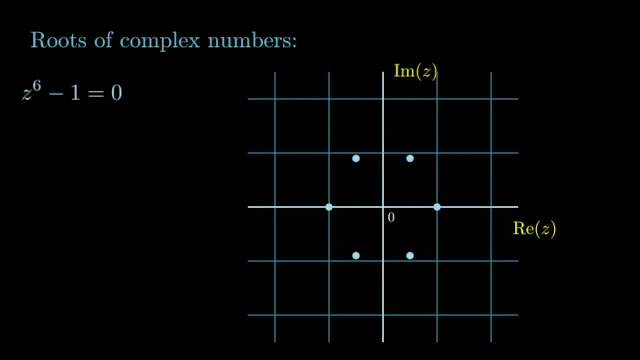 roots are depicted here, And if we look at the six roots of 1, we have this picture. So to actually calculate these roots of the complex numbers and find them on the Argand diagram, we're going to use Demwav's theorem. So suppose that z to the n is written in polar. 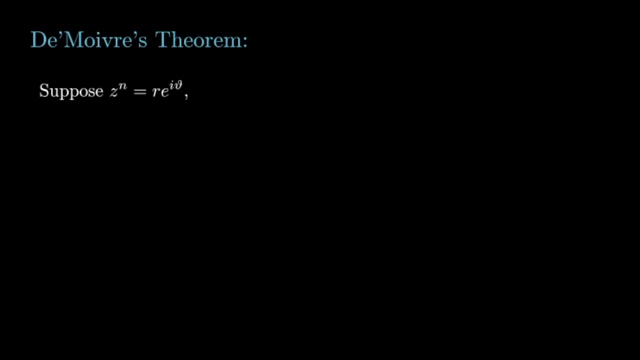 form as r, e to the i theta. Then Demwav's theorem says that the nth root of this complex number is given by taking the nth root of the modulus. So we're going to take r to the 1 over n And we will divide the argument by n, And then, since there will be n roots, we need to cycle. 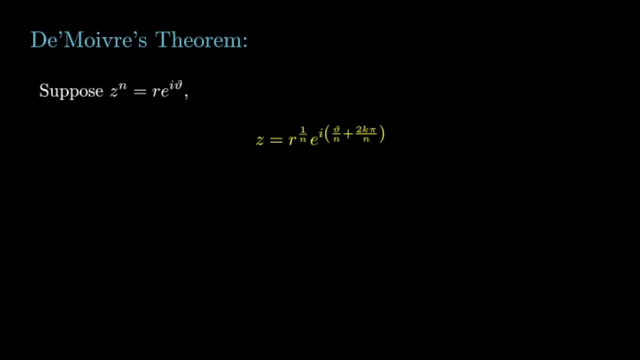 through. So we'll have this 2k pi over n factor. Let's look at an example. So find the three roots of i. So what we'll do is we'll write i in polar form, which we can write i as e to the i pi on 2.. 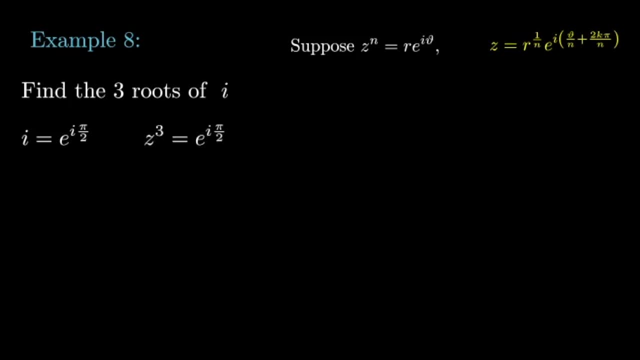 Then we want to solve the equation: z cubed is equal to e, to the i pi on 2.. And the kth? how many are there? n, N? So we're going to do that Right. And then we want to set the ki at. 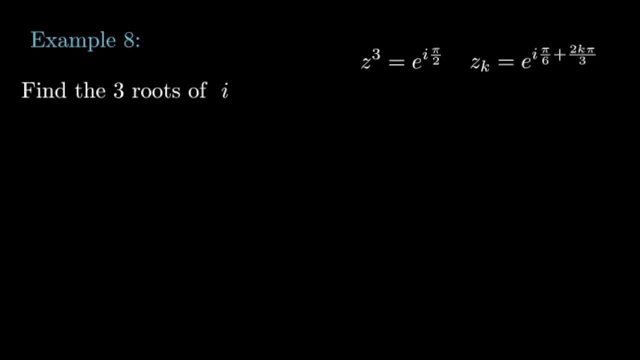 n. So we're going to do that first: m, Z, 2, pi on 3.. And so if we add these fractions together, pi on 6 plus 2, pi on 3 is going to be 5, pi on 6.. So we'll have e to the i, 5, pi on 6.. And if we take k equals 2, we'll find that z2. 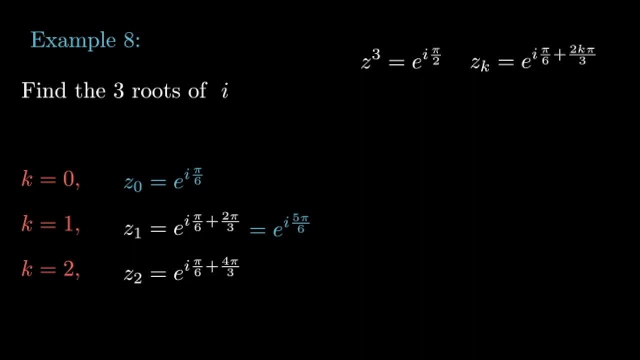 is e to the i pi on 6, plus 4 pi on 3.. And if we add these fractions together, we'll end up with e to the i, 9 pi on 6.. 9 pi on 6 simplifies to 3 pi on 2.. And so what we need to do is subtract. 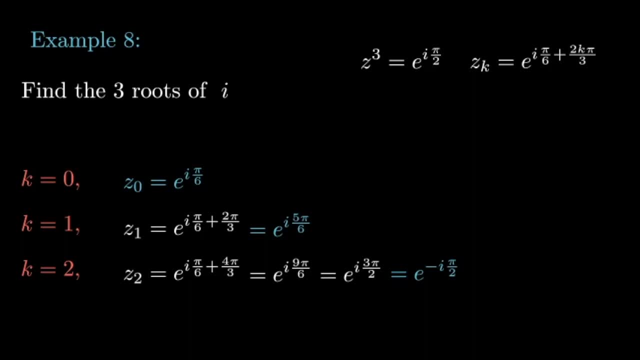 2 pi. In that case we see that 3 pi on 2 minus 2 pi is minus pi on 2.. And the final answer for z2 is going to be e to the minus i pi on 2.. Now, if we put these on a complex plane, 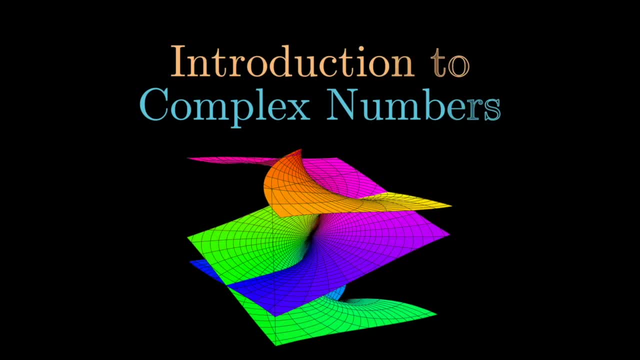 If you like the video, hit the like button. That'll do some fancy things with the YouTube algorithm to show this video to more people. I'm not going to ask you to hit the bell icon. I never hit the bell icon for anyone, even if I actually look forward to their content. A number of 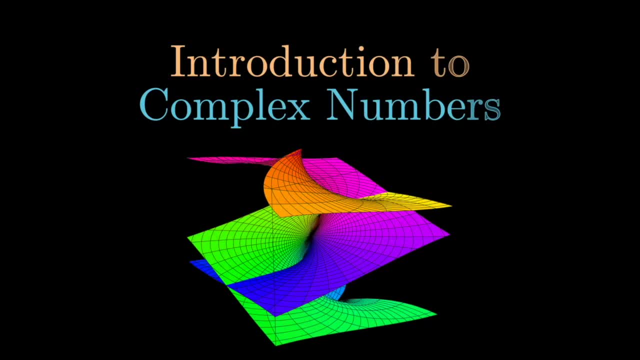 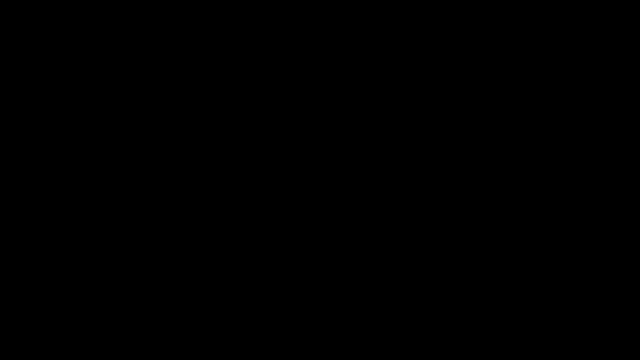 notifications will pop up every time I post a video. So if you like the video, hit the like button. I'll see you in the next video. Bye, See you in the next video. See you in the next video. See you in the next video.